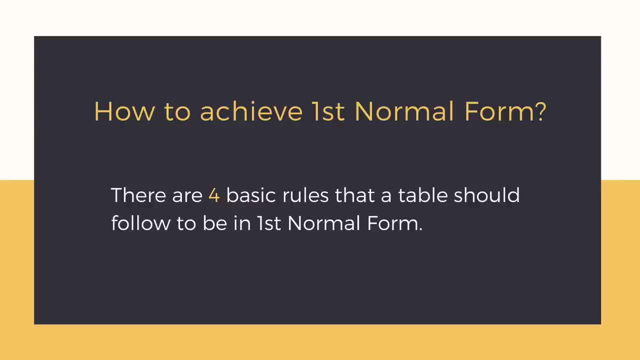 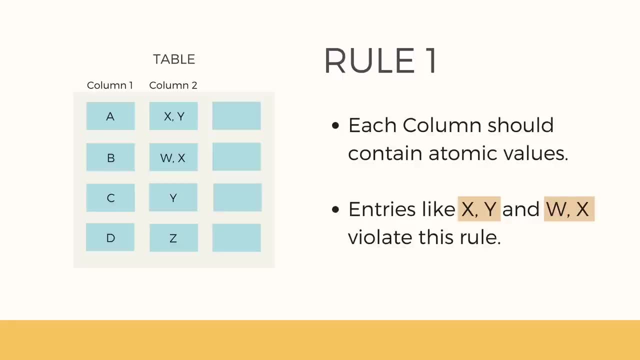 expects you to follow a few simple rules while designing your database, and they are: Rule number 1. Each column of your table must be single-valued, which means it should not contain multiple values. We will explain this with help of an example later. Let's see the 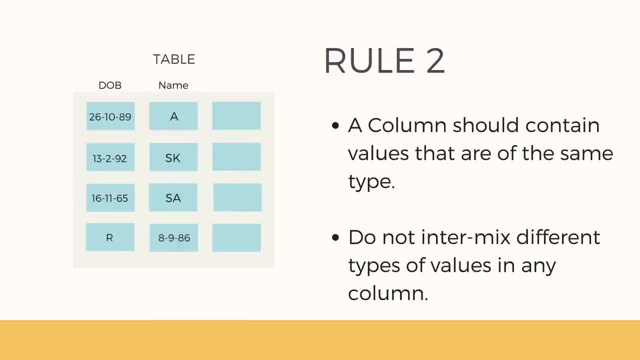 other rules, for now Rule number 2. This is more of a common sense rule. In each column the value stored should be of the same kind. For example, if you name a column date of birth to save date of births of a set of people, then you cannot or you must not save names of some of them in that. 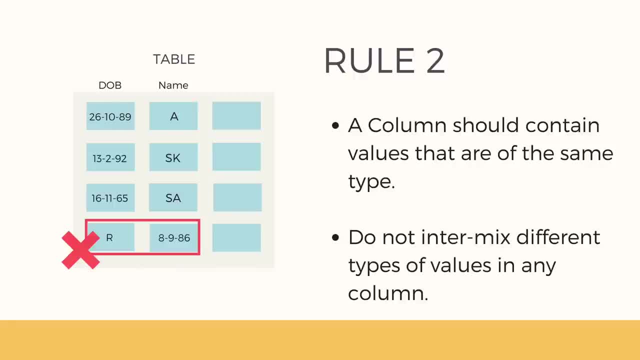 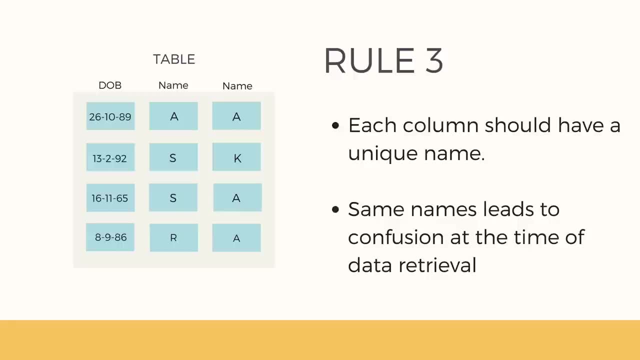 column along with date of births of others. in that column, It should hold only date of birth for all the entries or rows. Rule number 3 expects each column to have a unique name. This is to avoid confusion at the time of retrieving data. 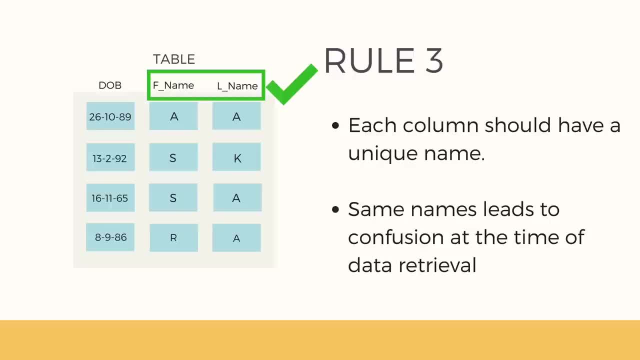 Rule number 3.. This is to avoid confusion at the time of retrieving data. If one or have same name, the DBMS system will be left confused. Rule number 4 says that the order in which you store the data in your table doesn't matter, Although all 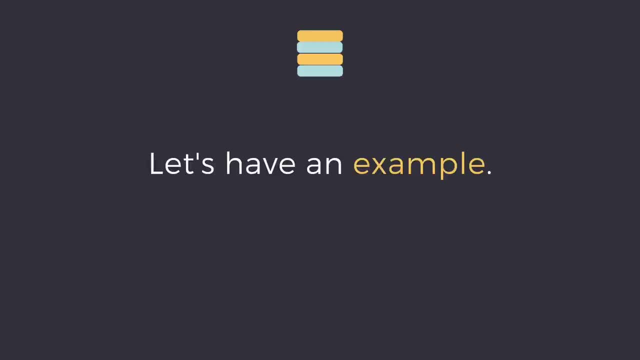 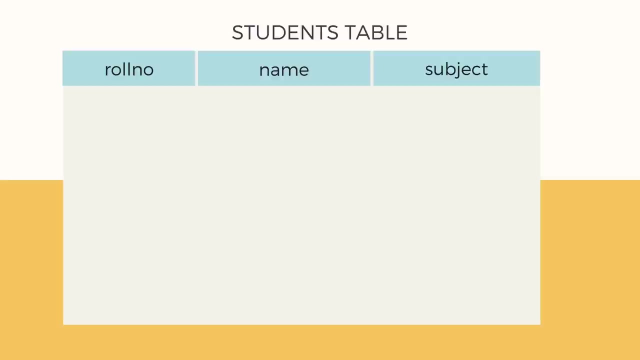 the rules are self-explanatory. still, let's take an example where we will create a table to store student data, which will have students role number, their name and the name of subjects they have opted for. So we will be creating a table with three columns. We can obviously have as many columns in a 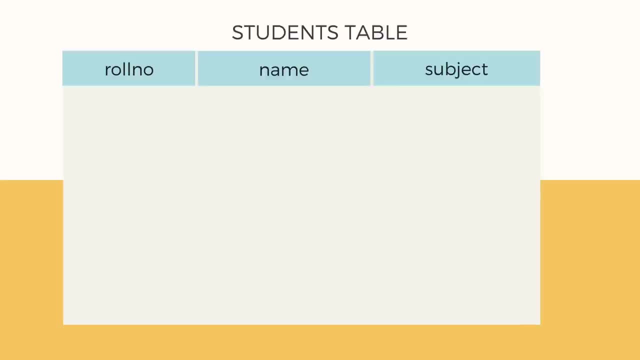 table as we want, but for our example we only need three. We will name the columns roll number, name, subject: let's add some data to our table. Now, with data added, a table already satisfies three rules out of the four rules: Auss, all our column. 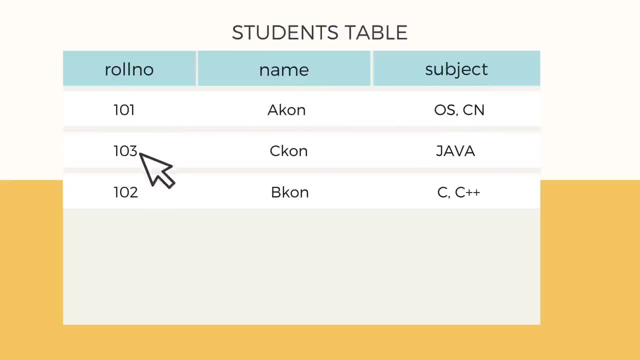 names are unique. we have stored data in the order we wanted to and we have not missed it. fixed different types of data in our columns, but out of the three different students in our table, two have opted for more than one subject and we have stored the subject names. 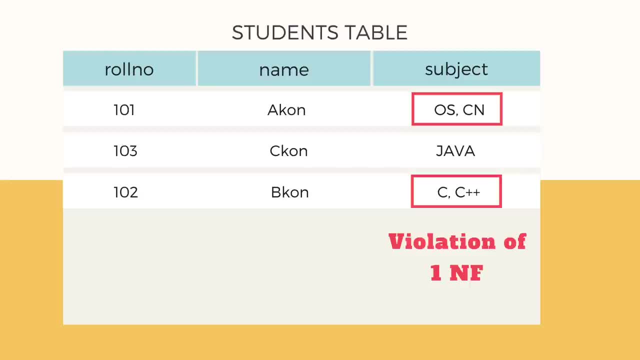 in a single column, but, as per first, normal form, each column should contain atomic values. now, how to solve this problem? it's very simple, because all we have to do is break the values into atomic values. by doing so, although few values are getting repeated, but values for